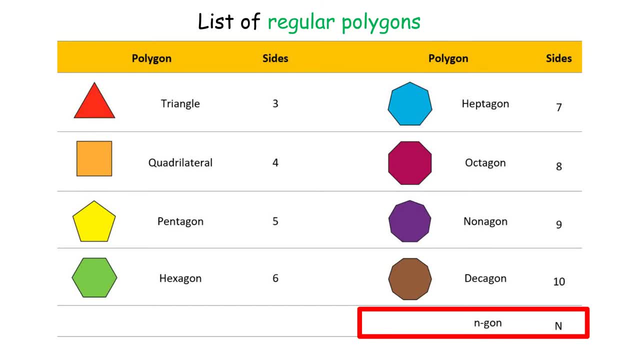 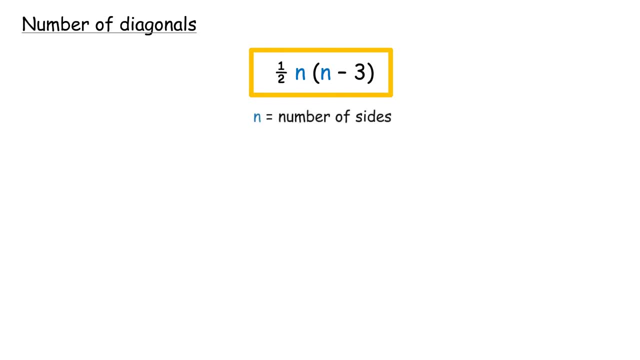 Decagon, ten sides And gon n sides. Number of diagonals equals half n times n minus three. where n equals number of sides, Number of diagonals for a triangle is zero. Number of diagonals for a quadrilateral is two. 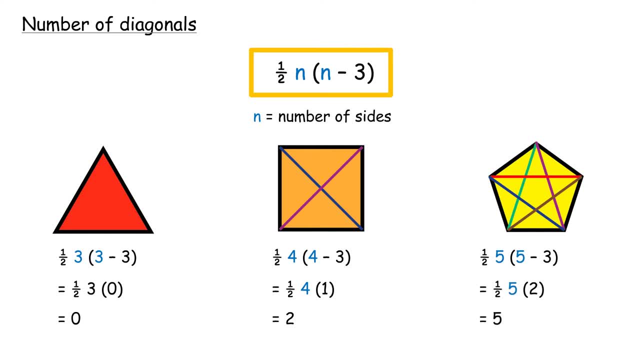 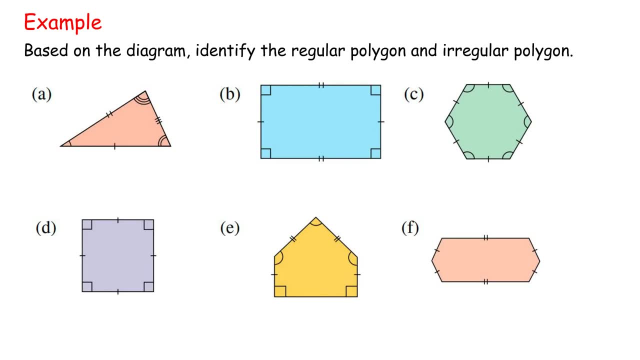 Number of diagonals for a pentagon is five. Example Based on the diagram: identify the regular polygon and irregular polygon. Solution: A- Irregular polygon. B- Irregular polygon. C- Regular polygon. D- Regular polygon. 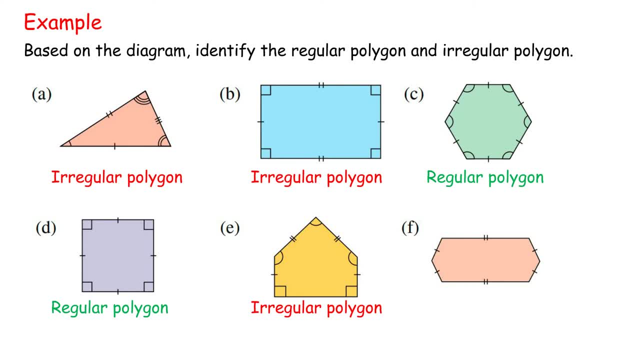 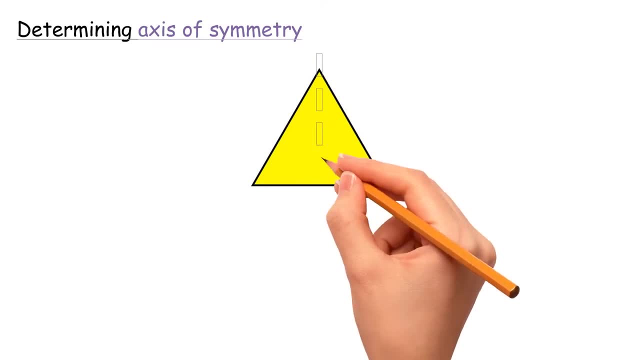 E- Regular polygon. F- Irregular polygon. Determining axis of symmetry: A line through a shape so that each side is a mirror image. When the shape is folded in half along the axis of symmetry, then the two halves match up. 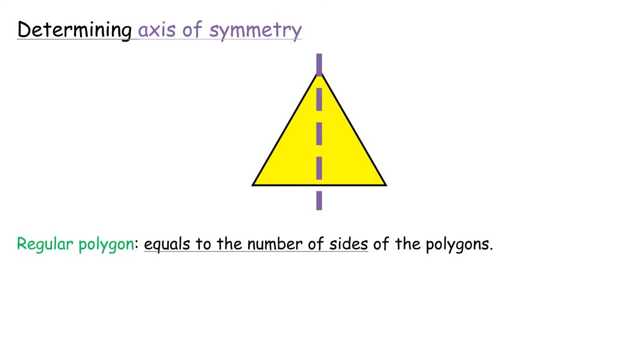 The number of axis of symmetry for a regular polygon is equals to the number of sides of the polygons. The number of axis of symmetry of irregular polygons should be explored using the folding method. Regular polygon, An equilateral triangle three sides, has three lines of symmetry. 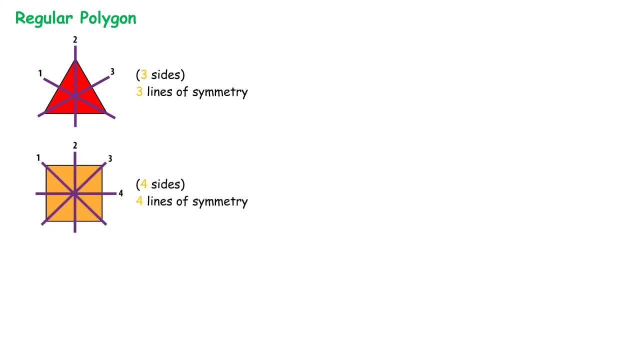 A square, four sides, has four lines of symmetry. A regular pentagon, five sides, has five lines of symmetry. Irregular polygon, Isocelles triangle has one line of symmetry. Scaling triangle has no line of symmetry. Rectangle has two lines of symmetry. 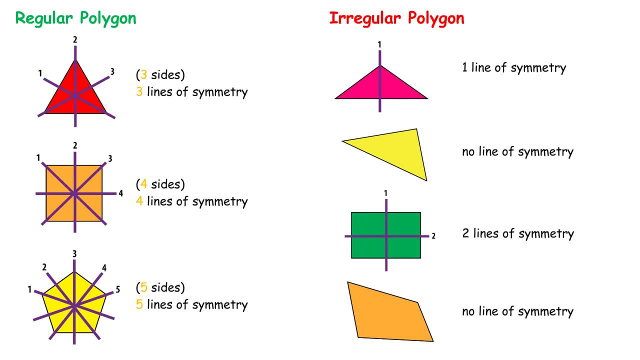 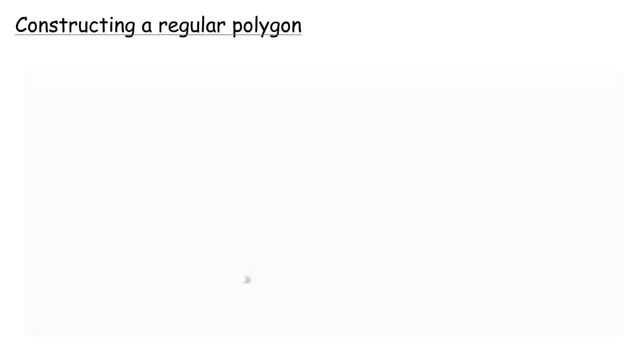 Irregular quadrilateral has no line of symmetry. Constructing a regular polygon Using geometry tools, Construct an equilateral triangle with the sides five centimeters A. construct a line, segment AB, with length five centimeters B. construct a curve with a radius five centimeters from point A. 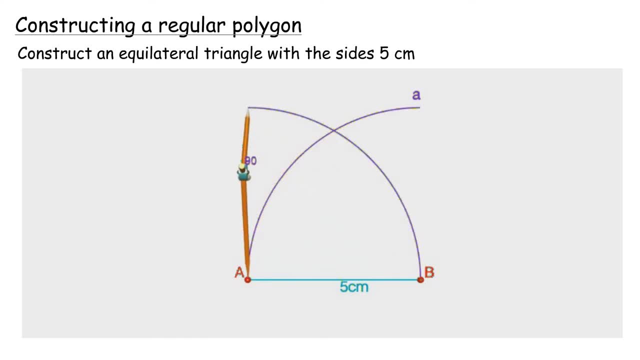 C. construct a curve with radius five centimeters from point B so that it intersects with the first curve. The intersection point is labeled C. D. draw a line from A to C and from B to C. An equilateral triangle is created. 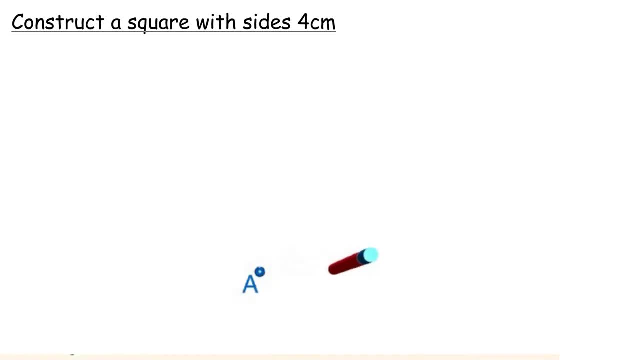 Construct a square with sides of four centimeters. Construct a line, segment AB, with a length four centimeters. A, shape it and manage it by a Roger to Z formula. A is trained to draw with circumstances A and B is trained to draw with situations C. 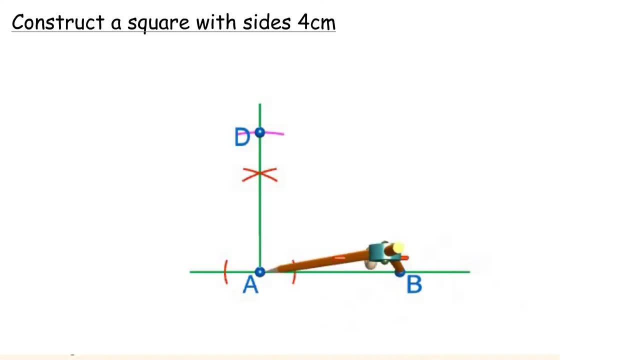 A is trained to draw with situations B and C. philosophically, A is trained to draw with circumstances A and C with circumstances B, B and D, so that both the curves intersect. The intersection point is labeled C. Construct a regular hexagon with sides 3.5 centimeters. 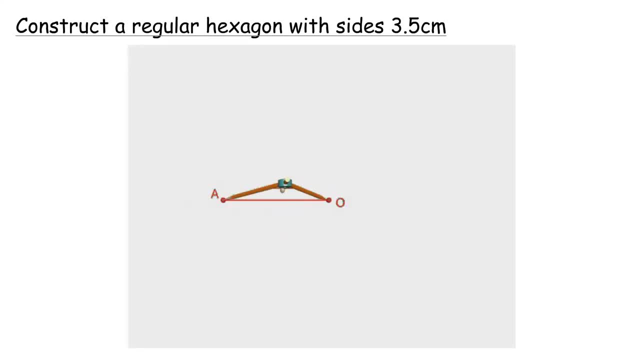 Construct a circle with a radius of 3.5 centimeters. Mark one point at the circumference and label it A. Construct a curve with radius 3.5 centimeters from A and label it B. Construct a curve with a distance 3.5 centimeters from B and label it C. 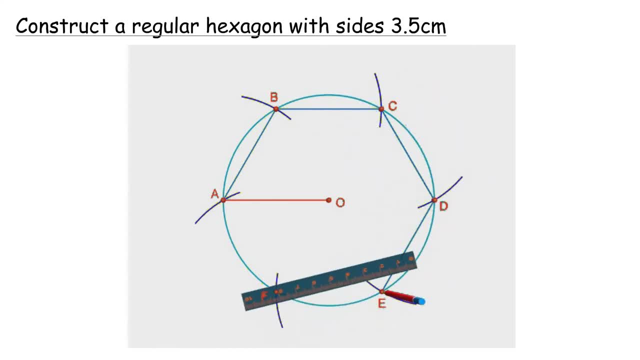 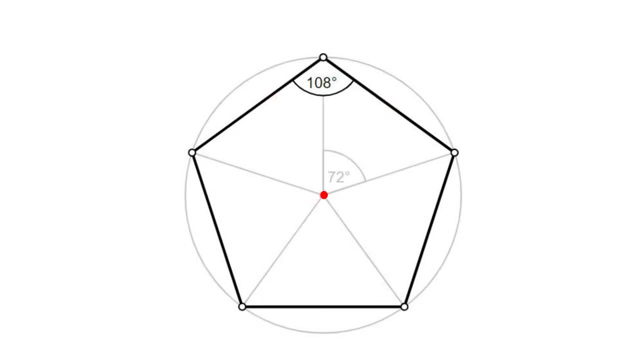 Repeat the steps until F. Draw a line ABBCCDDEEFFA to form a regular hexagon. Regular polygons can also be constructed by dividing the angles at the center of a circle according to the number of sides. 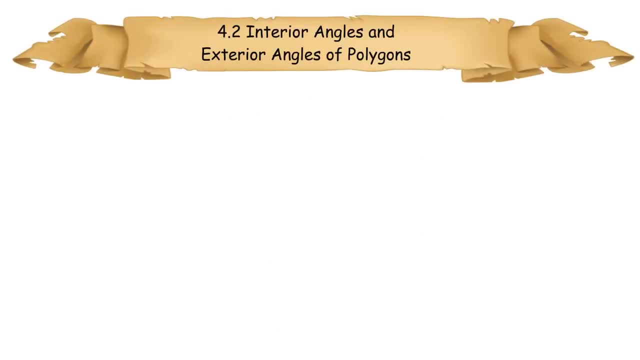 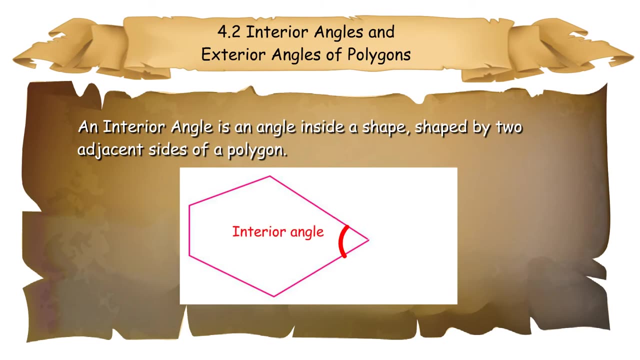 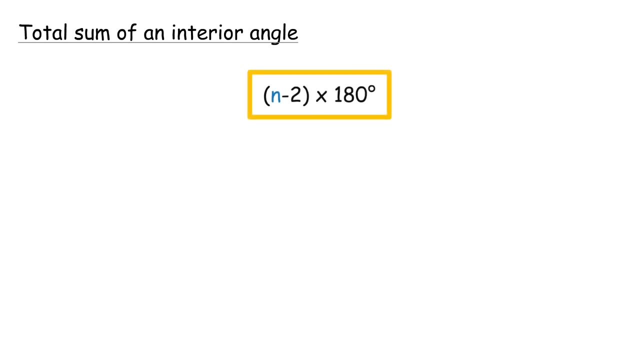 4.2. interior angles and exterior angles of polygons. An interior angle is an angle inside a shape Shaped by two adjacent sides. sides of a polygon. interior angle plus exterior angle equals 180 degrees. the total sum of an interior angles of a polygon equals n minus 2 times 180 degrees, where n is number of sides. 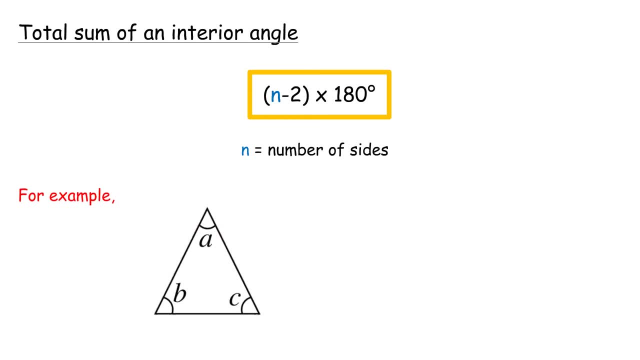 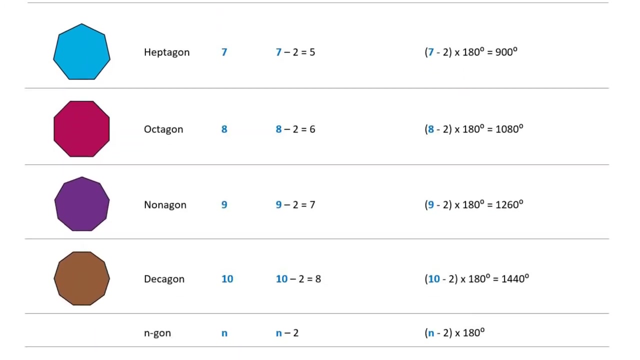 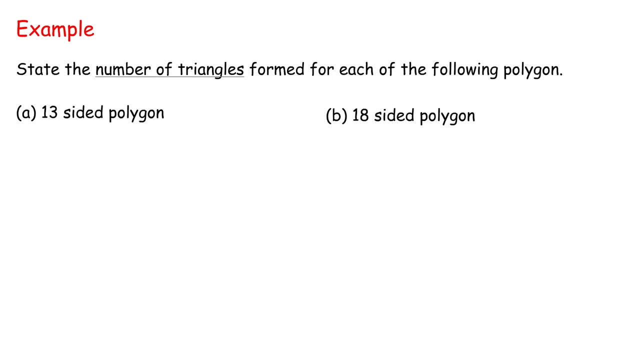 for example, the sum of an interior angles of a triangle equals 3 minus 2 times 180 degrees equals 180 degrees. a plus b plus c equals 180 degrees. the polygons and interior angle. some measures are as below. example state: the number of triangles formed for each of the. 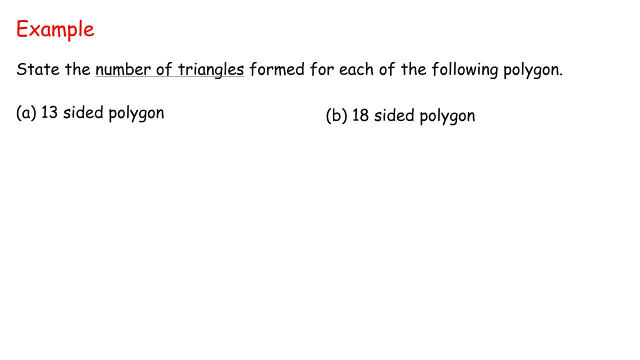 following polygon solution: a- 13-sided polygon number of triangles equals 13 minus 2 equals 11. b- 18-sided polygon number of triangles equals 18 minus 2 equals 16. example: calculate the value x for the following solution: a total sum of interior. 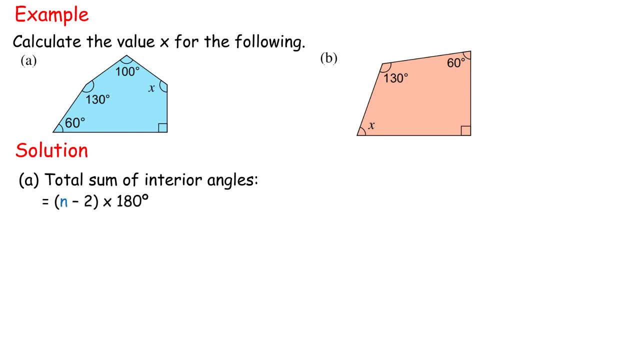 angles equals n minus 2 times 180 degrees equals 5 minus 2 times 180 degrees equals 540 degrees. x plus 100 degrees plus 130 degrees plus 60 degrees plus 90 degrees equals 540 degrees. x plus 380 degrees equals 540 degrees. x, equals 540. 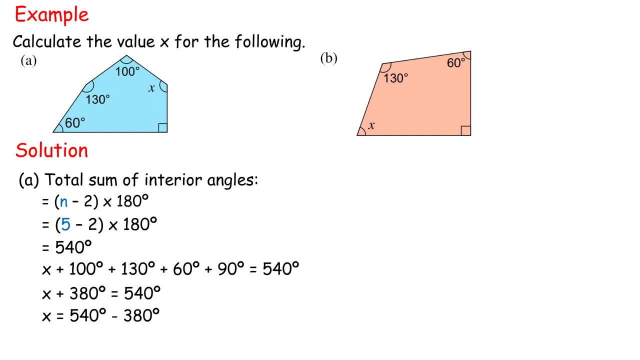 degrees minus 380 degrees equals 160 degrees. the total sum of interior angles equals: and minus 2 times 180 degrees equals 4 minus 2 times 180 degrees equals 360 degrees. x plus 130 degrees plus 60 degrees plus 90 degrees equals: 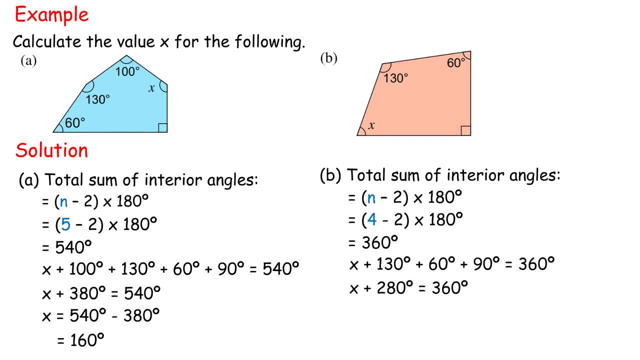 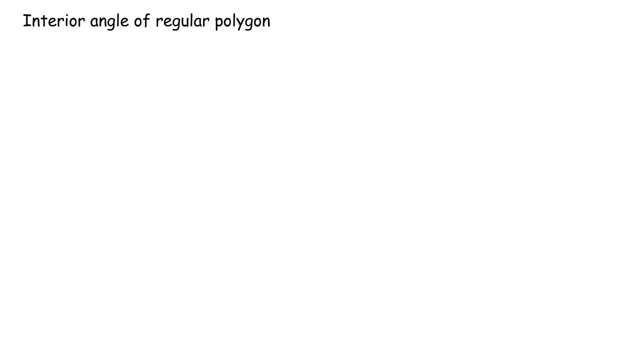 360 degrees. x plus 280 degrees equals 360 degrees. x equals 360 degrees. minus 280 degrees equals 80 degrees. interior angle of regular polygon: E equals and minus 2 times 180 degrees divided by n. example: calculate the value of the interior angle. 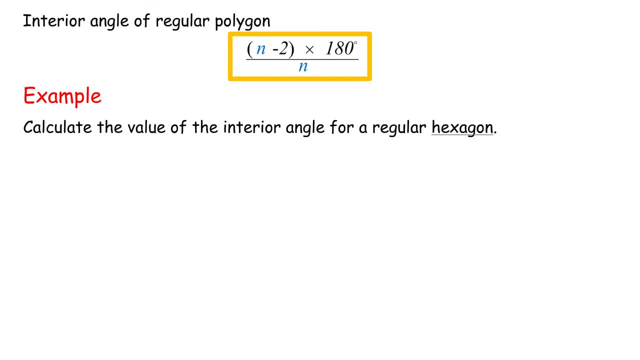 for a regular hexagon solution. number of sides of regular hexagon: n equals 6. total sum of interior angles: equals and minus 2 times 180 degrees equals six. minus t times 180 degrees equals four times 180 degrees equals 720 degrees. plywood below symbol. 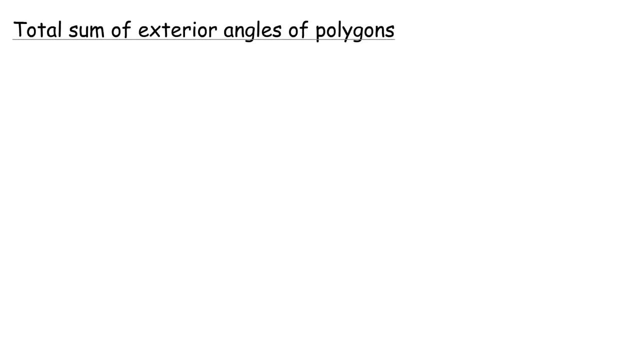 Now let's break continuously this ganze recursion data to completekapitalize. one side of the polygon is extended. it is the supplementary angle to the interior angle of the adjacent side. the total sum of exterior angles of a polygon is 360 degrees. exterior angle of a regular polygon equals 360 degrees divided by number of side n. example a: calculate the value. 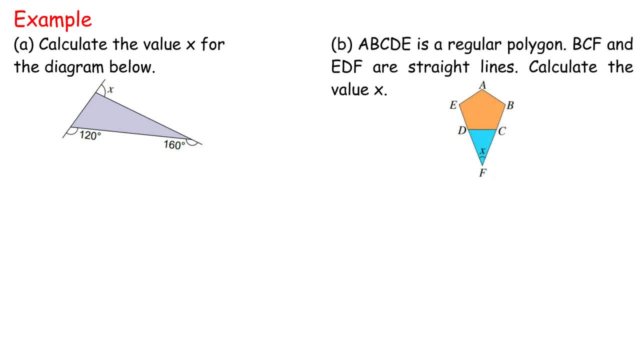 x for the diagram below b. in the diagram below a, b, c, d, e is a regular polygon. b, c, f and e, d, f are straight lines. calculate the value x solution: a total sum of exterior angles equals 360 degrees. x plus 160 degrees plus 120 degrees equals 360 degrees. 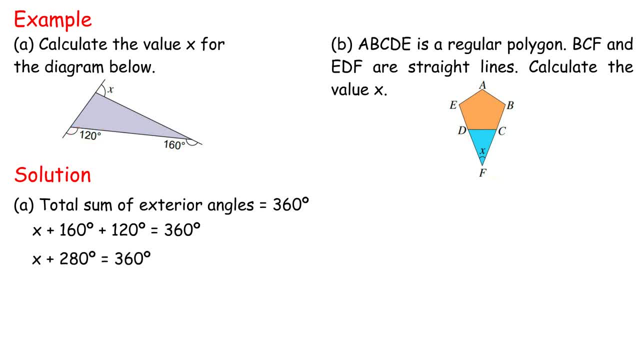 x plus 280 degrees equals 360 degrees. x equals 360 degrees minus 280 degrees equals 80 degrees. b fcd equals 360 degrees. divided by 5 equals 72 degrees. x equals 180 degrees minus 72 degrees minus 72 degrees equals 36 degrees.